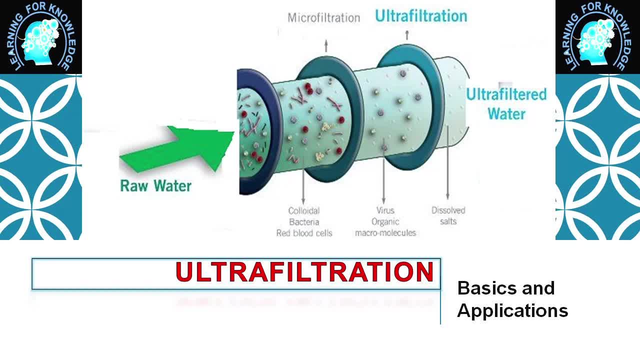 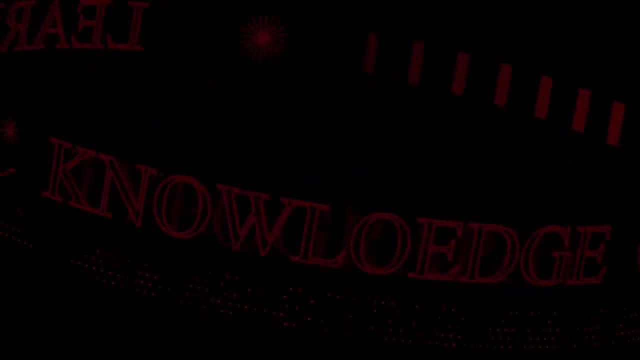 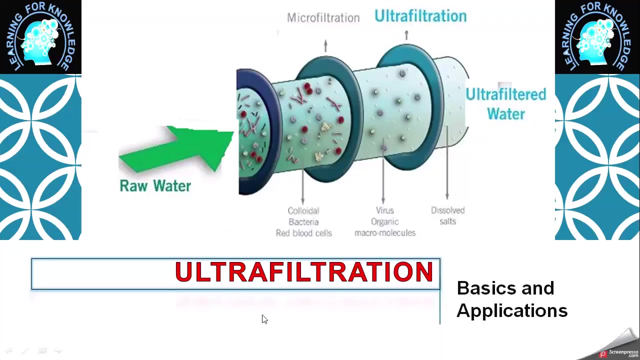 or nanofiltration, in which we will use a membrane but the size of the pore is different from other techniques, So we will describe this technique, its basic and applications only in this video. What is ultra filtration Now? ultra filtration basically a pressure driven membrane. 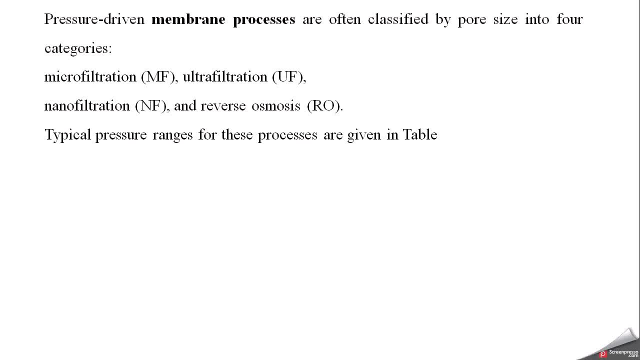 process And the pressure driven membrane process, which have different categories, are often classified based on their pore size, And there are four major types based on membrane process and pressure driven process. Number one is micro filtration, which is abbreviated by MF, Ultra filtration, UF, which will be 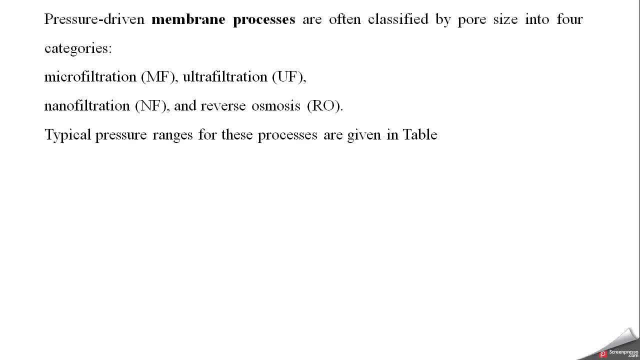 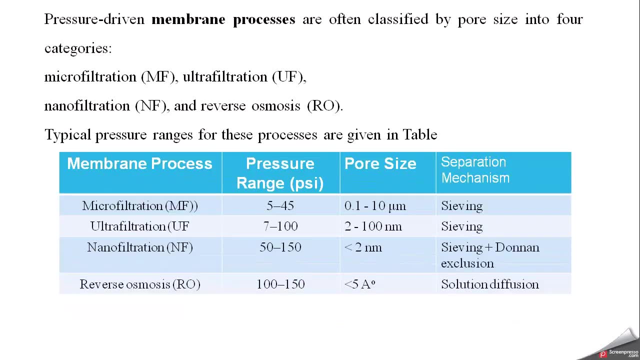 described in this video: Nanofiltration, NF, and reverse osmosis, which is RO. So typical pressure ranges for these processes are given in this table. You can see that if we move from micro filtration to reverse osmosis- reverse osmosis processThe pressure ranges which is given in the second column, that 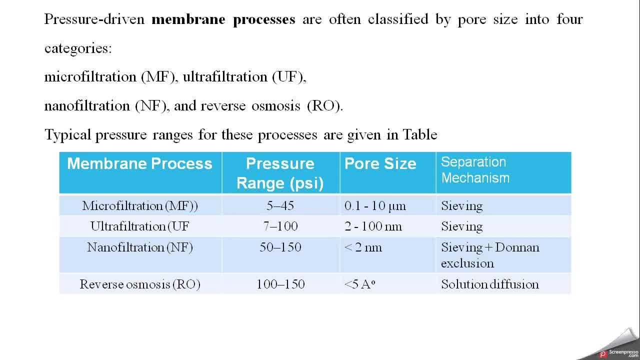 is start from a very low pressure of 5 to 45 psi and then if we move towards higher site reverse osmosis, its pressure is increase up to 150 and similarly the pore sizes in micro filtration is greater as, which is around 0.1 to 10 micron, and in reverse osmosis it's around 5 angstrom or 0.5. 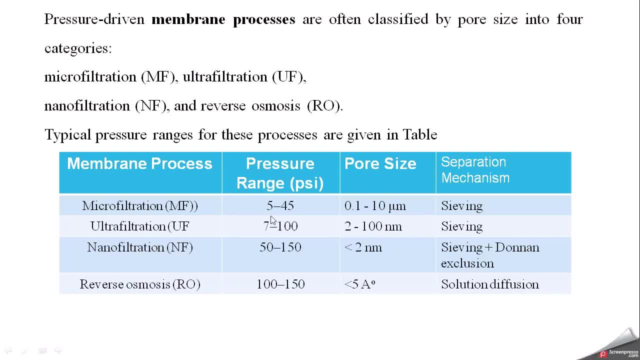 nanometer. so you can see that as the pressure increases now, the pore size decreases, or vice versa, as the pore size decreases, we have to increase the pressure, and this is basically the pressure driven membrane processes. however, the separation mechanism in all these techniques are slightly different. if we look or focus on micro filtration, ultra filtration, then it is purely based 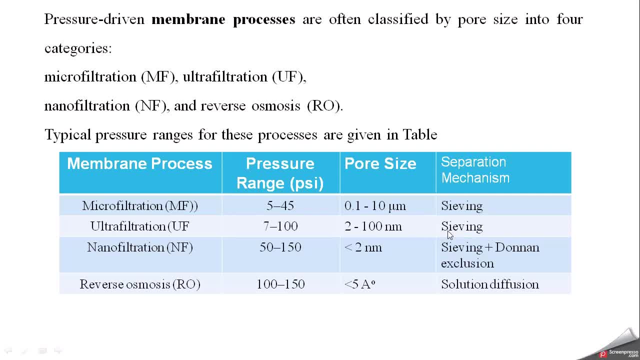 on sieving, that is the particle, which are have less size than the pores, they will pass from the membrane and other, which have higher size, stop at the membrane surface and in nano filtration. this is a combination of sieving plus exclusion, donon exclusion and fourth one which is reverse osmosis. basically, this is based. 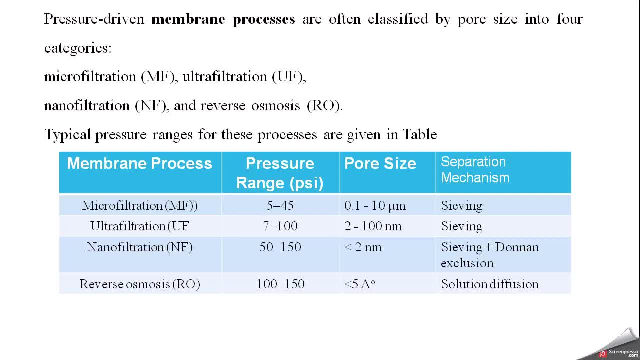 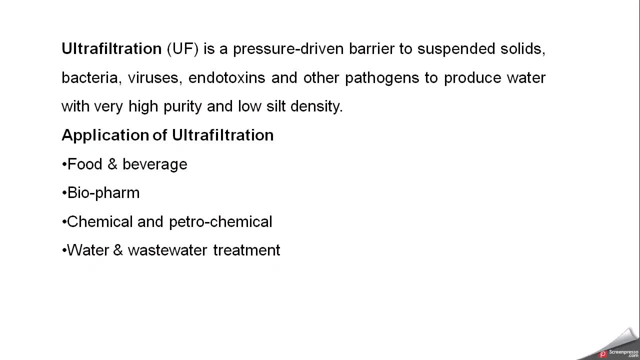 on diffusion process, chemical potential and other things which, like some of these things I have explained in other videos, related with reverse osmosis. now we come towards the ultra filtration, which is also abbreviated as UF, is a pressure driven barrier to solids back which are now suspended solids, bacteria, viruses, endotoxin and 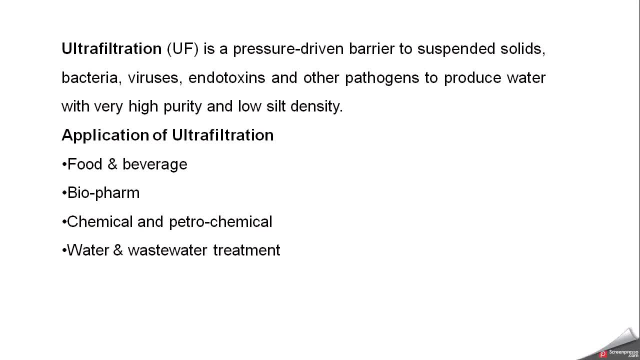 other pathogens to produce water with very high purity and low silt density, which has low silt density. so basically, by applying the pressure and we have a membrane in the path which is based on point 1.01 and 0.01 micron. then this: 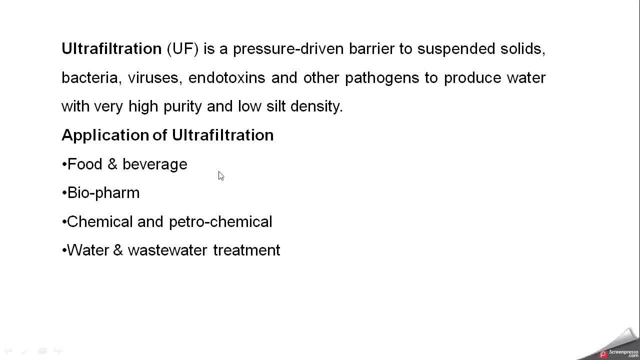 technique is UF and it's we can find the applications of this technique in food and beverage, biopharmaceuticals, chemical and petrochemical waste and wastewater treatment. so if we look where we have a particle size in the range of some few microns, like 0.01 micron, we can apply this and the pores will stop the impurities which 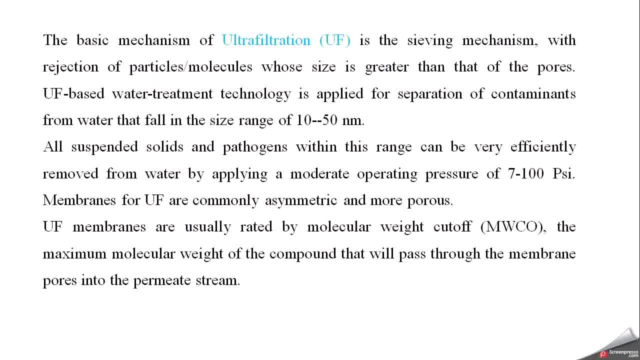 come in this range. so basic mechanism, if I explain this UF is the sieving mechanism with rejection of particle molecules whose size is greater than that of the pores. those molecule which are greater in size will stop on the on this membrane surface and cannot pass through the pores. so you have based water. 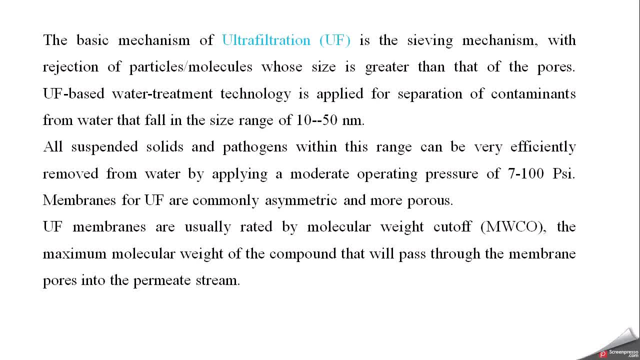 treatment technology is applied for separation of contaminants from water that fall in the size range of this 10 to 50 nanometer. so all suspended solids, pathogen viruses and other impurities within this range can be very efficiently removed from water by applying a moderate operating pressure of seven 200 psi, depending upon 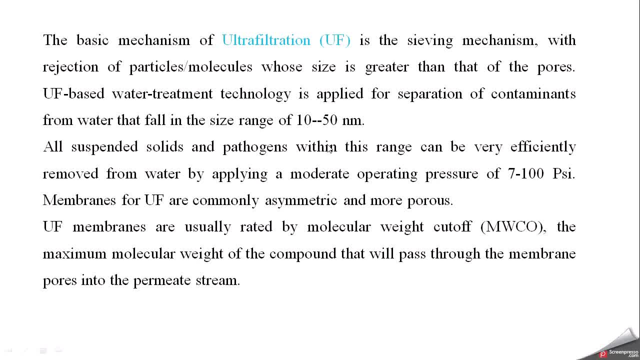 the impurities. so membranes for UF are commonly aerated membranes and the other membranes for UF are commonly aerated membranes. so membranes for UF are commonly aerated membranes and they can be removed from the water by applying a asymmetric and more porous and usually rated by a molecular weight cut off, which is abbreviated: 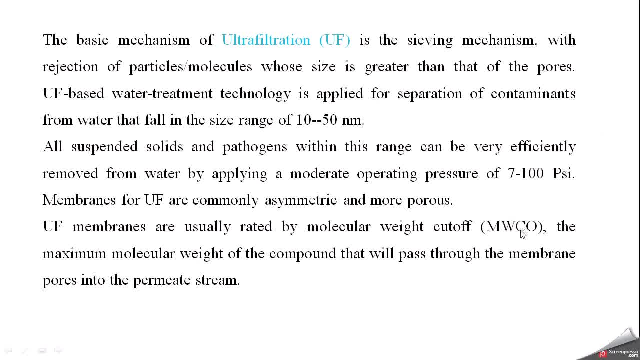 by MWCO molecular weight cut off The maximum molecular weight of the compound that will pass through the membrane pores into the permeate stream. So whenever we you can say, categorize or give the properties of UF, then basically it is quoted that this much size or maximum, this much size of the particle or impurities or 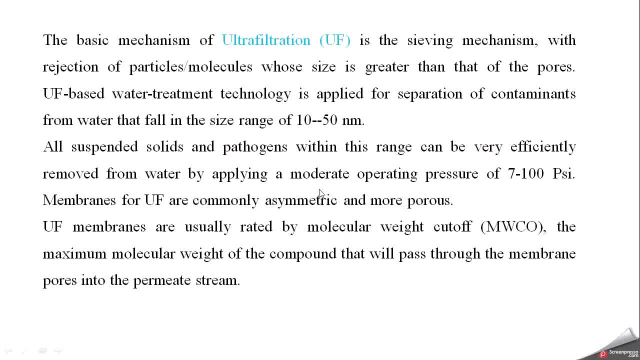 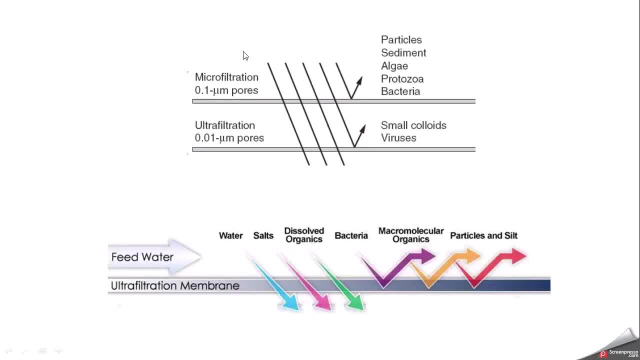 molecules will be stopped on the surface of the membrane, So abbreviated by MWCO. Now, this is. from this figure you can see that in microfiltration, approximately 0.5 micron pore size, the particle which will be stops are sediment, algae, protozoa, bacteria of. 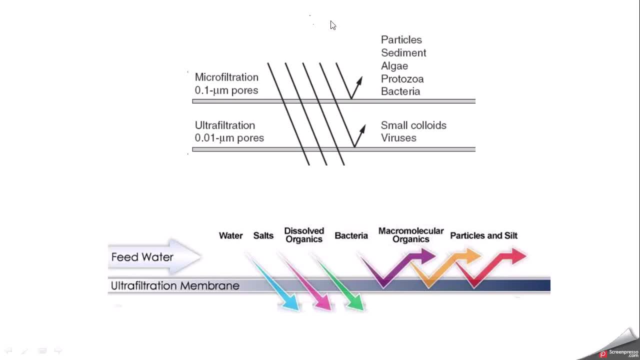 this size, So these particles will stop and remaining will be passed. Now, after microfiltration, we have a ultrafiltration and the pore size is 0.01 micron, and small colloidal viruses and other bacteria of smaller size will stop on the surface and rest of 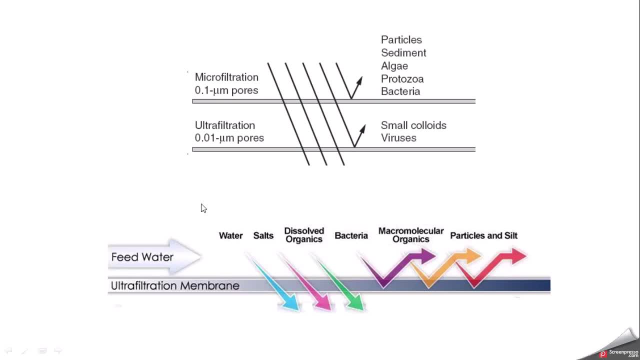 the dissolved solids will pass through this. This is another way of looking towards ultrafiltration: that water, salts, dissolved organics will pass from this membrane. However, bacteria, molecular, macromolecular organics, particles and silt who have a size. 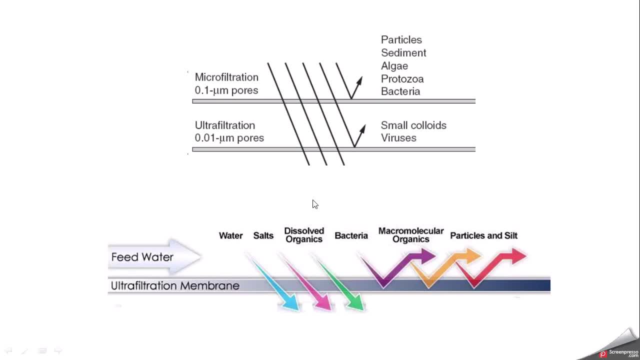 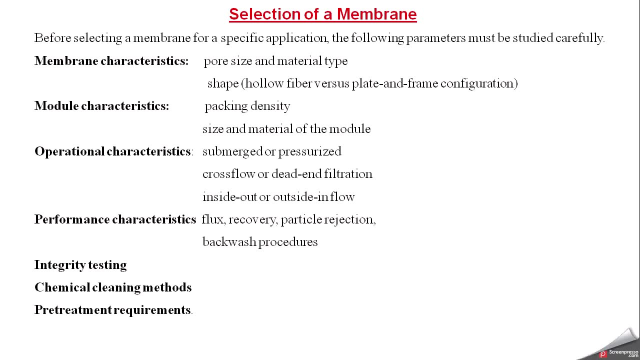 of greater than 0.01 micron, they will be stopped on the surface of this ultrafiltration. Now, if we want to select a membrane, then what we need to understand we have to look on what type of parameters. First of all, membrane characteristic, that is, pore size and material type. 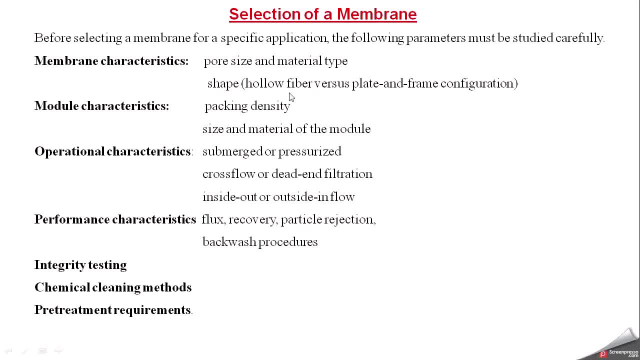 That is, what is the material of the membrane and its shape, like hollow, fiber plate, and end frame configuration, whatever types. Second is module characteristics: packing density, size and material of the module, operational characteristics and other important thing that whether membrane can be submerged or 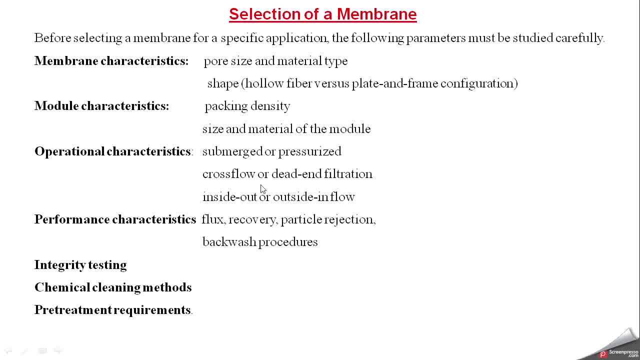 pressurized cross flow or dead end filtration, inside out or outside in flow, Depending upon your requirement. you will consider these things And then performance characteristic. very important that what is the flux recovery of the purified water, particle rejection, backwash procedure so that you can easily clean the membrane. 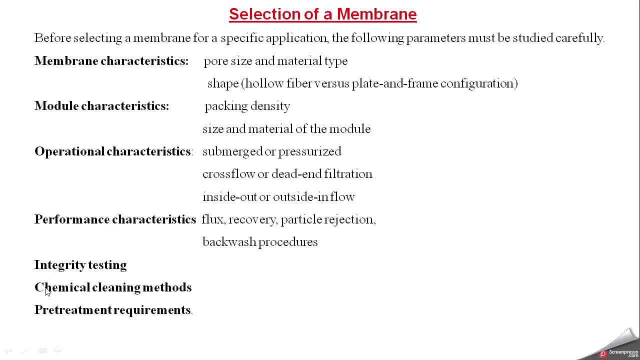 when it is clogged, Integrity testing, chemical cleaning methods for cleaning purposes and pretreatment requirement, if any. These things, these parameters or these aspects must be considered before you are going to select a membrane. In this video I am focus very general and basic things, not going into detail aspects. 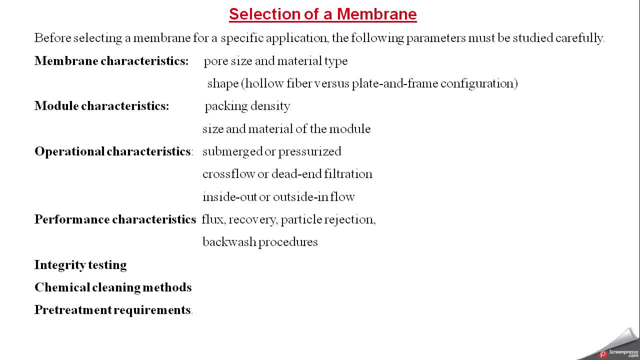 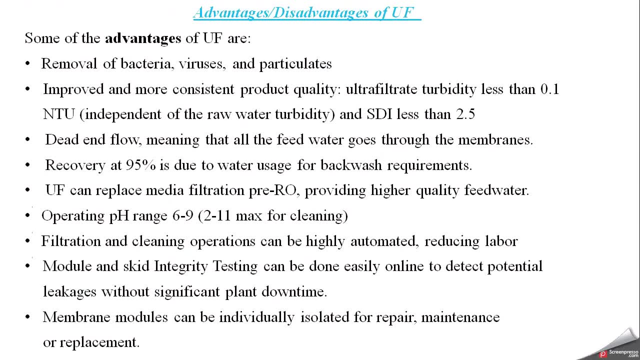 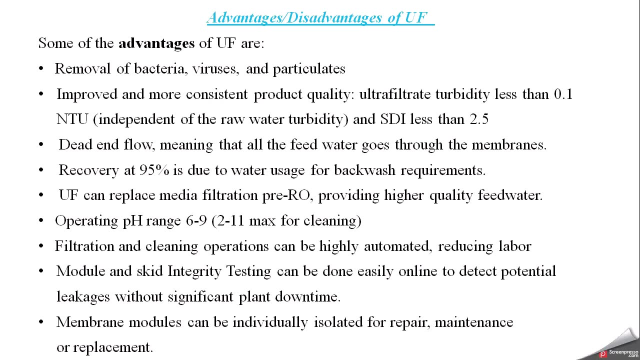 maybe if we will get time and in the next videos we will explain all these things one by one. So after this- now there are some- we are focus on advantages and disadvantages of ultrafiltration. So first one, filtration. here on this page we have summarized some of the advantages of uf, so obviously, removal. 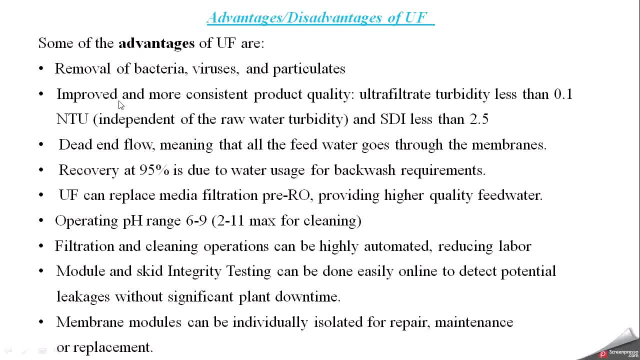 of bacteria, viruses and particulates. improved and more consistent product quality: same or consistent quality of the water we will get using ultra filtrate and ultra filtrate turbidity less than 0.1 ntu and sdi less than 2.5. however, if you are getting higher turbidity or higher sdi, then you 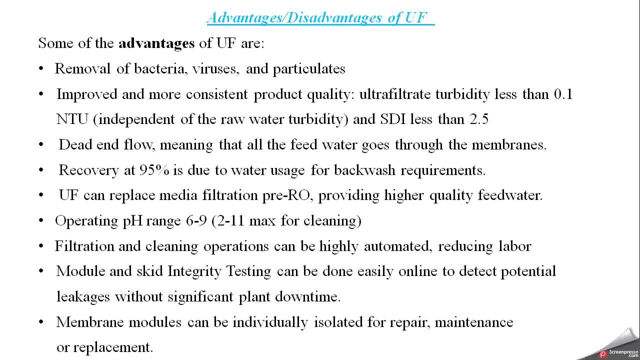 should consider that your process is not going in a correct way. dead end flow. if you are using dead end flow, meaning that all the feed water goes through the membrane, no wastage, so recovery at 95, this is due to reason that five percent of the remaining water is normally used. 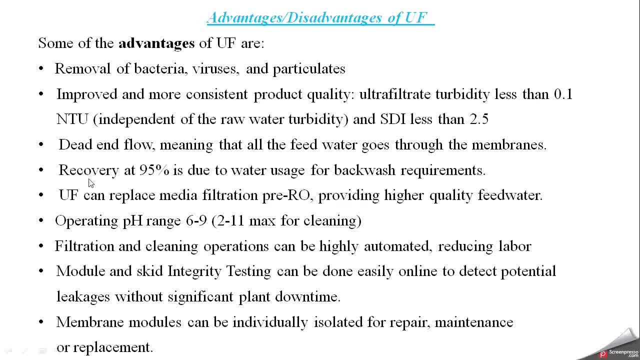 in during the backwash which will be wasted. so very high efficiency or recovery. uf can replace media filtration pre-ro like multimedia carbon filters and other sand filters etc. which are used as a pre-treatment of ro. if you place install uf, there's no need to use those accessories. 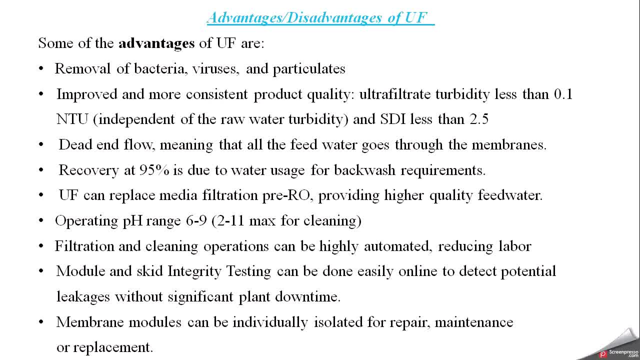 because uf is providing much higher quality of the water. operating ph range normally 6 to 9, but it can withstand in 2 to 11 ph range. because of cleaning sometimes you use acids and bases. so basically membrane material must withstand up to within the range of 2 to 11 ph. filtration and 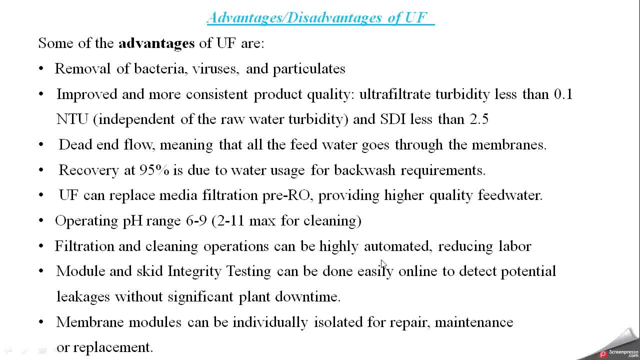 cleaning operations can be highly automated and reducing the labors. similarly, and medull and skid integrity testing can be done easily online and membrane medull can be individually isolated. very good aspect- operation aspect- that if you have a like 4 or 6 membrane installed, then if you have a problem in one membrane you can isolate without stopping. 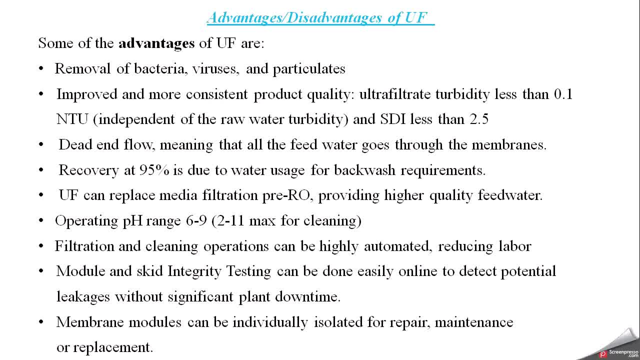 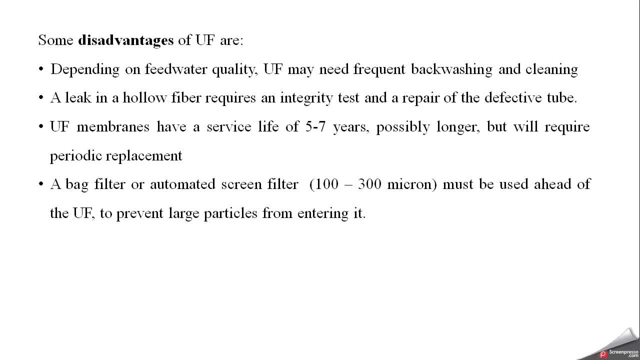 your process. you can isolate that membrane and your process will continue with rest of the membrane and you can repair the isolated membrane. then there are some disadvantages of uf. not big deal. depending on feed water quality, uf may need frequent back washing and cleaning, so this is not the disadvantage. basically, this is some lacking. 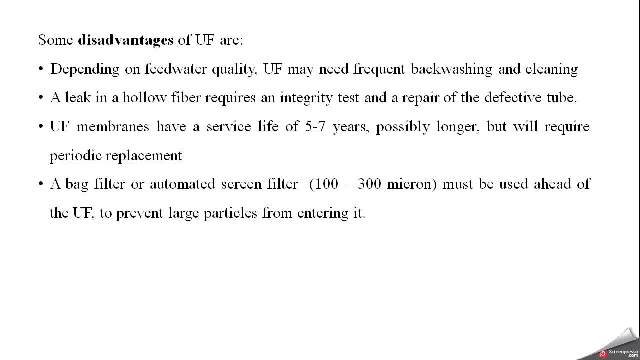 but it is also providing another thing: that if you have a dirty water and uf will clean it better way but downtime will increase due to its back washer. cleaning leak in hollow fiber require an integrity test. if there is some leak then you have to test, or the complete membrane, whether it can withstand with your pressure and other things. 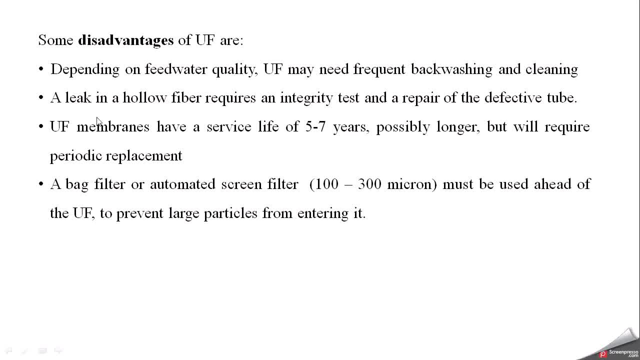 and repair of the defective tube. so UF membrane have a service life of 5 to 7 years depending upon this use. it may be increased or reduced depending upon the your operating, your operation methodologies. water, a bag filter or automated screen filter must be used that there is must. 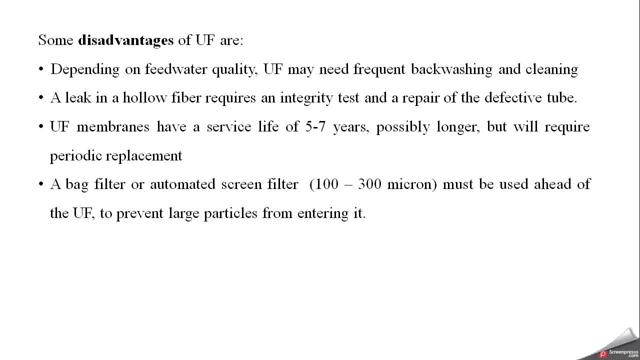 be a filter before this UF. so a big particles: instead of choking or clogging more frequent the UF, they will stop one step behind the UF. so by removing the big particle you can increase the efficiency of UF and prevent the leakage or damaging of the UF membrane. these are slightly at one disadvantages, but 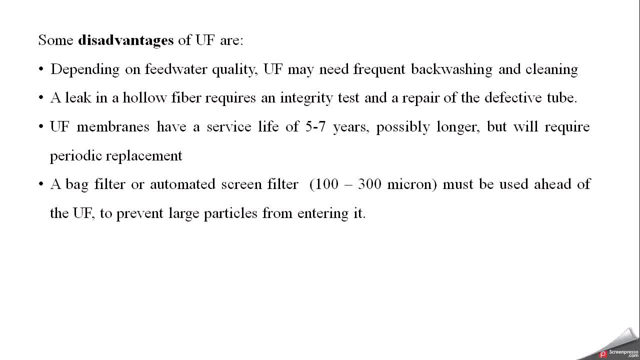 advantages of using UF are much more and greater than disadvantages. so this technique must be applied in in the pharma industry for removal of the micron sized particles in water and wastewater treatment. so, and this is also this use in the pre treatment of the reverse osmosis. 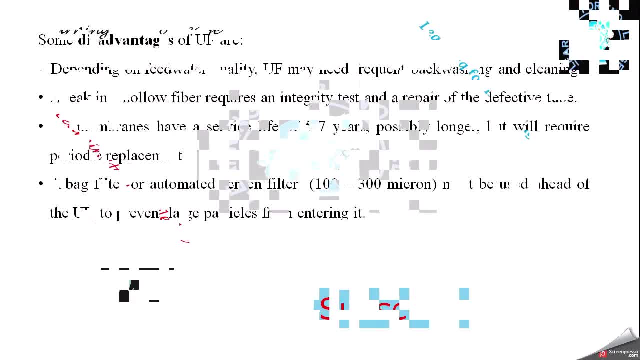 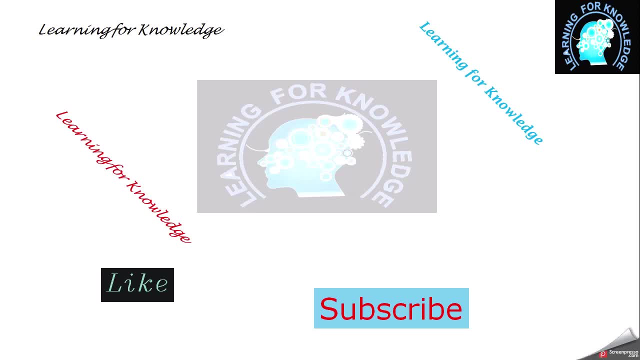 you plants. so this is about basics and advantage- disadvantages of ultra filtration. I hope you like this and we will provide you some more knowledgeable videos in the future. thank you very much. 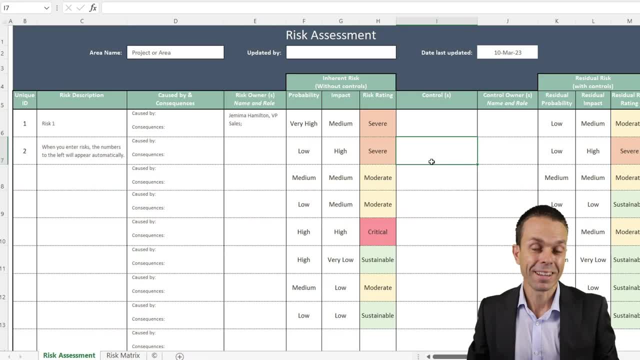 Hi everyone, this one is something absolutely fantastic. It's a risk assessment and if you work in risk or around risk, or in projects or even in a business that needs to measure risk, this is absolute gold and it's the best risk template that I have ever come across and I use. 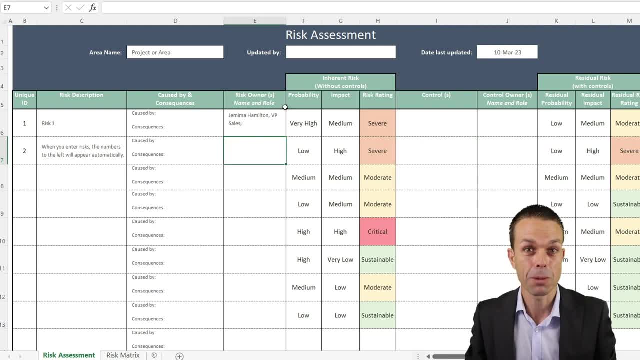 on a daily basis. There's a lot of different parts to this risk assessment and we're going to go through all of them to create it for yourself, if you want to. But long story short, as part of any risk and risk assessment. you've got your risk descriptions, you've got your. what are they? 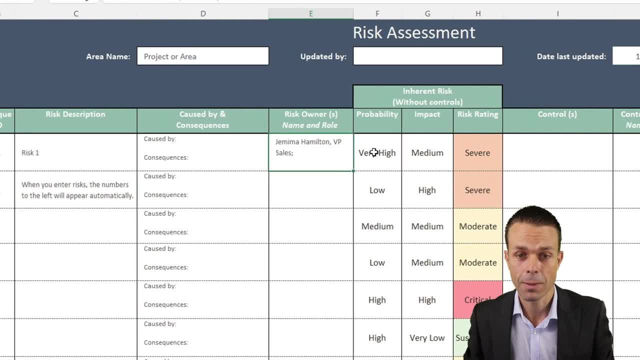 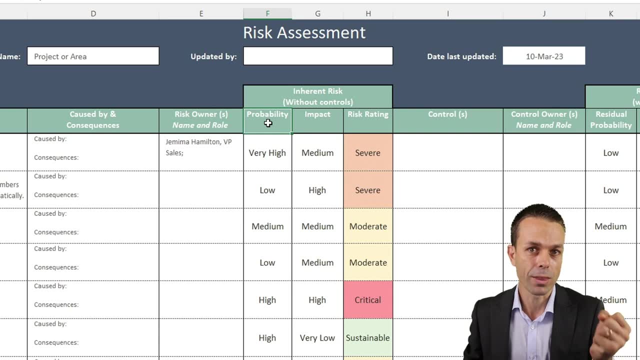 caused by and what are the consequences of them and who owns that risk. But then, most importantly, we've got the probability and impact, And for any risk we want to multiply the probability by the impact and that will give us our risk rating. So this particular sheet actually does. 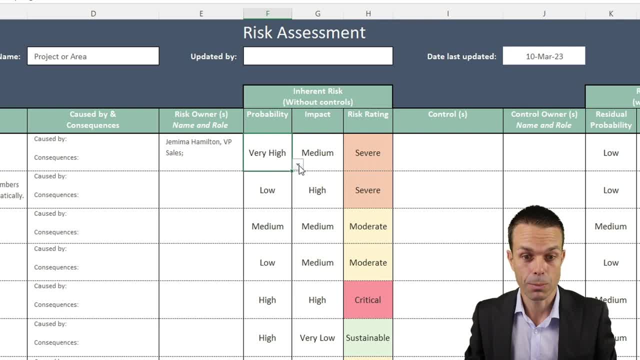 that automatically For us and what we do, as an example, is, if we select from a drop down, maybe it's a medium probability or, and you know, this could be a percentage as well And you can change it and we'll show you how to change it as well. But let's say the impact, when it happens is is really low, very.